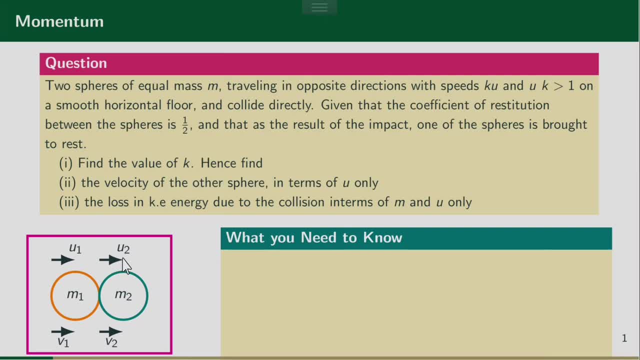 circles and their masses are m, M1 and m2.. Above, I have the values for their initial velocity and below I have the values for their final velocity. Now, in order to answer this problem, there are a couple of things that you need to know. The first thing you need to know is the law of conservation of linear momentum, which 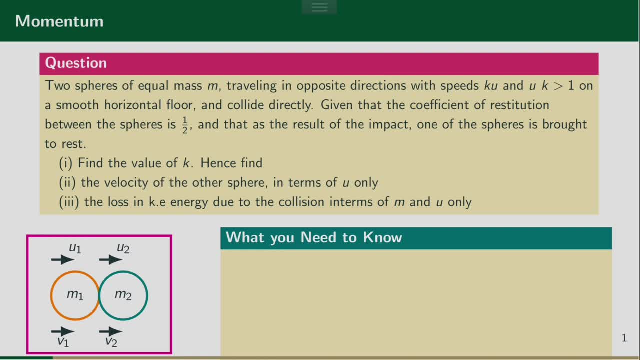 states that when two objects interact, the momentum before collision is always equal to the momentum after collision, provided no external force acts on them. How can we translate that mathematically? We can write it as the momentum of the first object, which is m1, multiplied by u1.. We add it to the momentum of the second object, which is m2. 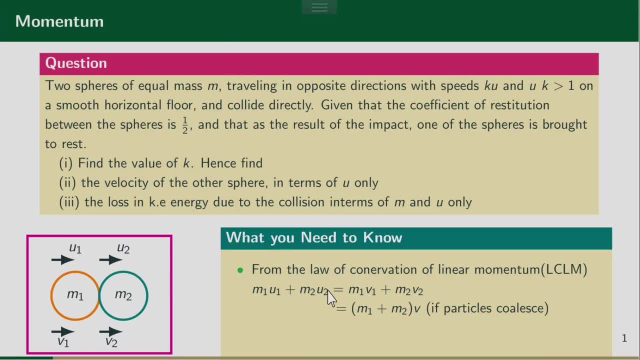 multiplied by u2.. The sum of these two momentum gives you the initial momentum of the object. Now, to obtain the final momentum, we just take their masses and we multiply by their final velocity and add them. So mathematically is how the law can be written. but in some cases, after the impact, some particles may stick together. 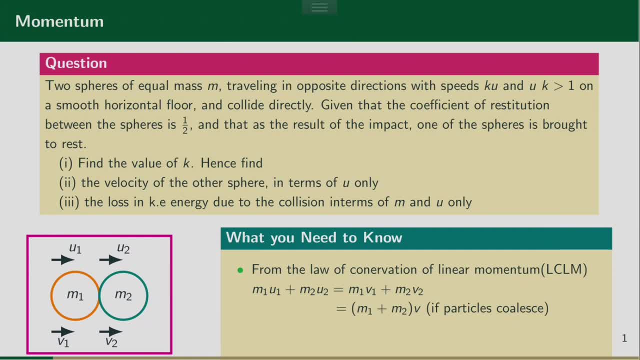 as one and move together. so they say the particle has coalesced. so in the case where they coalesce, then the momentum after collision will be the sum of their masses multiplied by that common velocity. so we'll be having m1 plus m2 multiplied by v, where v is a common velocity with which they 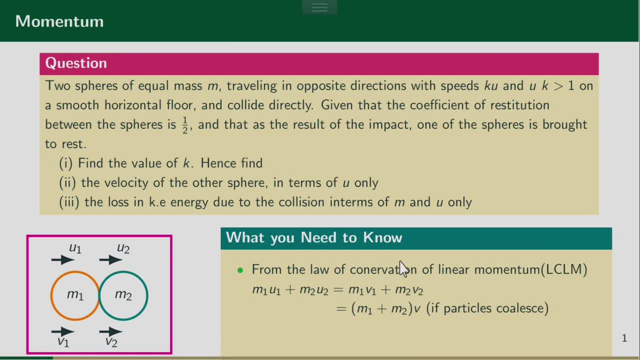 move after the impact. now, the second thing that we need to know is newton experimental law, and the law states that that the ratio of the speed of separation to the ratio of the speed of approach is a constant. that means when two objects interact, you can find the ratio of the relative velocities. 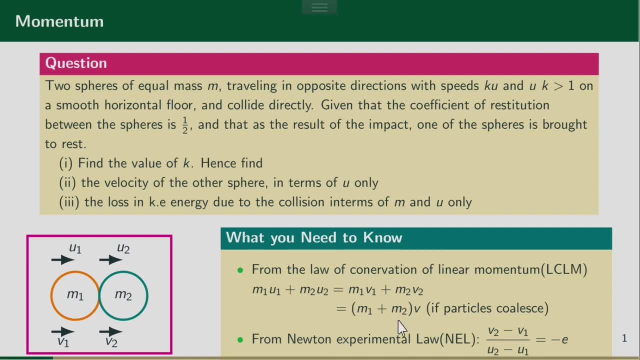 of approach to that of separation and mathematically it can be stated as: v2- take away v1 divided by u2- take away u1 is equals to negative e. in some books you can see: v2 minus v1 divided by u1 minus u2 is equals to positive e, but both of them represent the same. 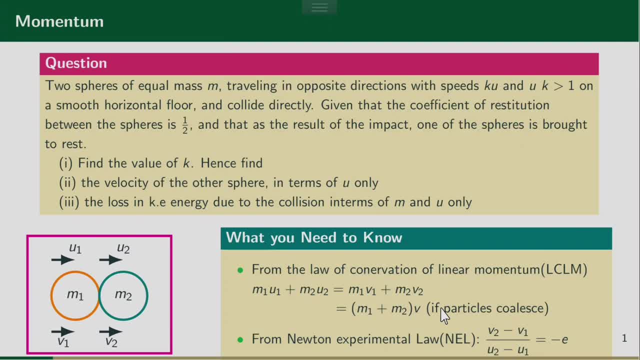 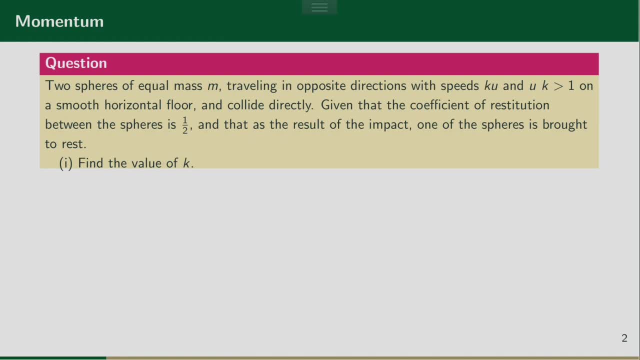 mathematical equation. now, with this being said, let's move on and answer the question. now i am going to concisely draw a diagram and represent the information from the. so here we have the diagram. we were told that two spheres of equal mass m, so that is why their masses. 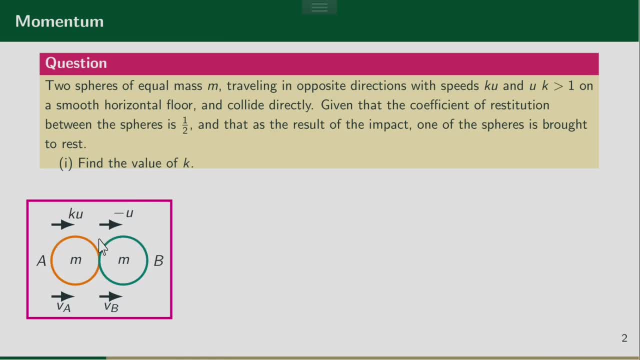 are all m and i've called the first fair a and the second phase i've named it b, with speed, ku and u, and they say they're moving in opposite directions. so if i consider the right direction as positive, then the left direction would be negative. so above here i've written the speed of a as ku. 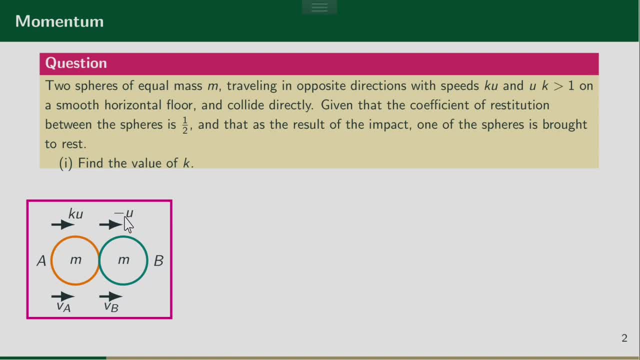 and that of b should be negative ku because a and b are moving in opposite directions. so if i had considered the left direction as positive, then this term ku will be negative and this term u will be positive. but in any case, make sure that you consider a reference. 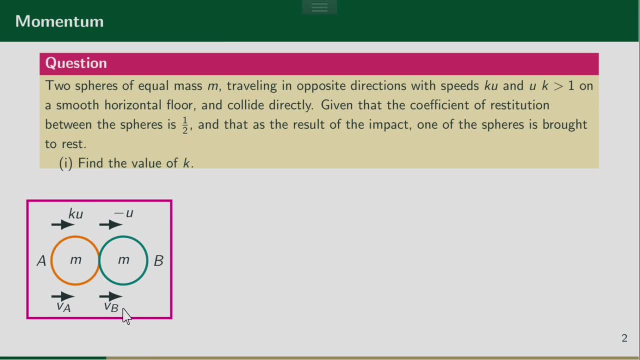 and solve to the end. now their final velocity is what i don't know. so let me call them v1 to stand for the final velocity of the first object, and v2 to stand for the final velocity of the second object or or of object b. now we have been told that let's find the value of k, but there's one. 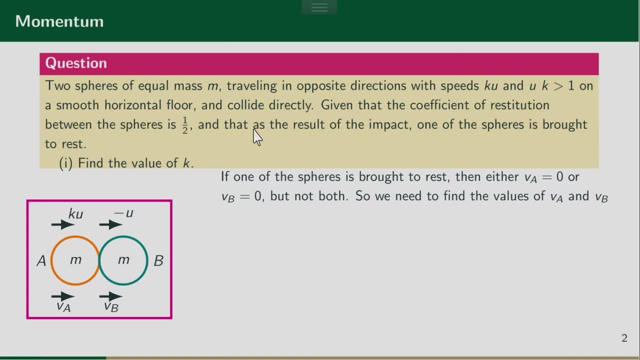 important information from the question. we have been told that after impact, one of the spheres is brought to rest. so one of the spheres is brought to rest. we don't know. and also in the question we have been told that k is a value of the first object and v2 to stand for the final. 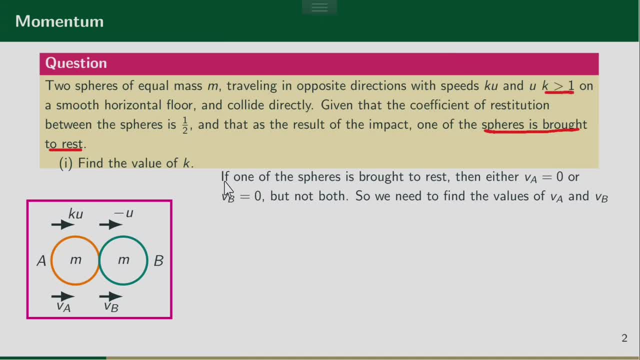 velocity of the first object and v2 to stand for the final velocity of the second object or or of object b. k is a value which is greater than one. so if one of the spheres is brought to rest, then either va is zero or vb is zero. that means either the final velocity of a is zero or that of b is zero. 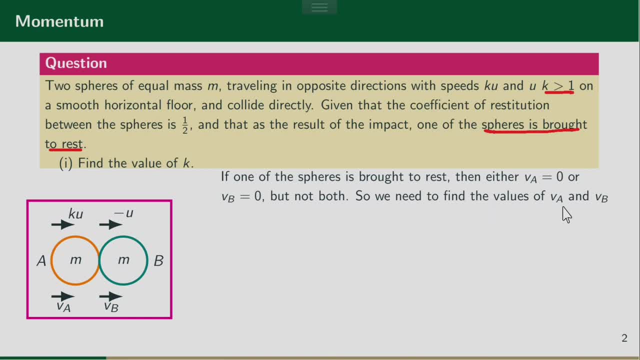 but not both of them. so we need to find the values of va and vb. by doing what? by making use of those two equations that we saw above. so, from the law of conservation of linear momentum, the momentum before impact will be m multiplied by ku. i add it to m multiplied by negative, u is equal to the. 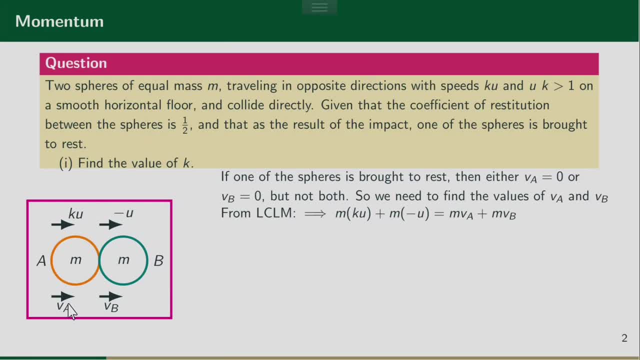 momentum of the space after impact, which is m va. i add it to m times vb. so notice that m is common to each term. so i use the equation n so you can know that n is between m and vb. foriren from size t and n is between space fit and stress after impact and n is between space fit and stress after. 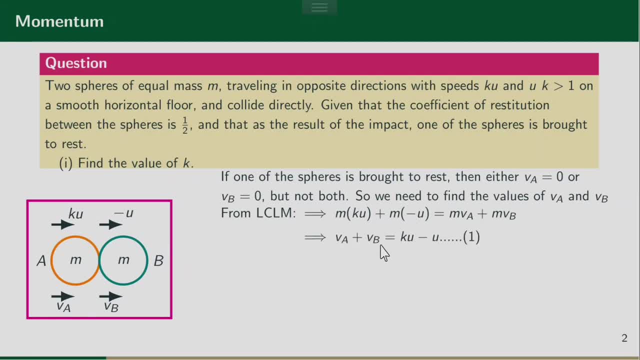 I can cancel out m from each of these terms, so I'll be having: v a plus v b is equal to k. u take away u. let me call that equation one. let me also use the idea of Newton experimental law and I'll have that from Newton experimental law. their speed of separation, which is v b minus v a, divided by 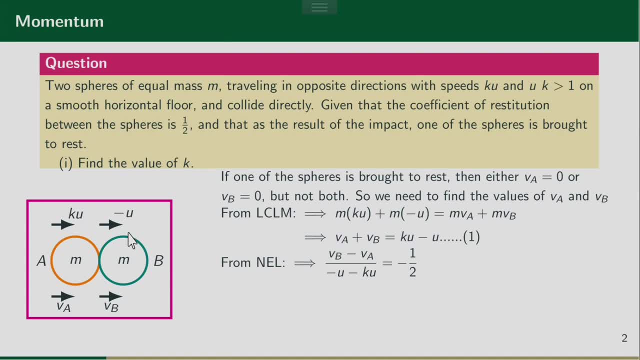 their speed of approach, which is negative. u minus k. u is equal to negative. e and e was given as half. now I can just multiply both sides by this denominator so that it cancels out and move on to the right hand side of the equation, and so I'll be having v b minus v. a is equals to negative. 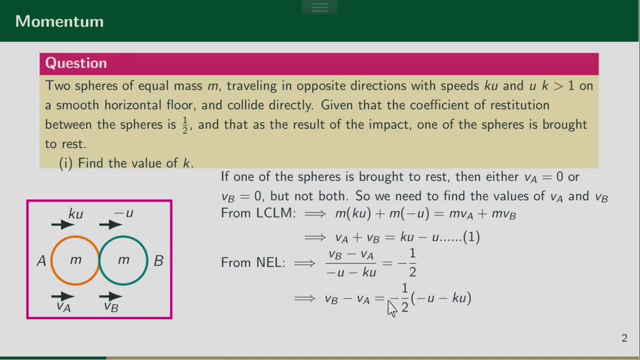 half into negative. u minus k, u, now negative, multiplies each of these terms and gives me a term, so So I'll now be having: VB minus VA is equals to positive U on 2.. I add that to positive KU on 2.. 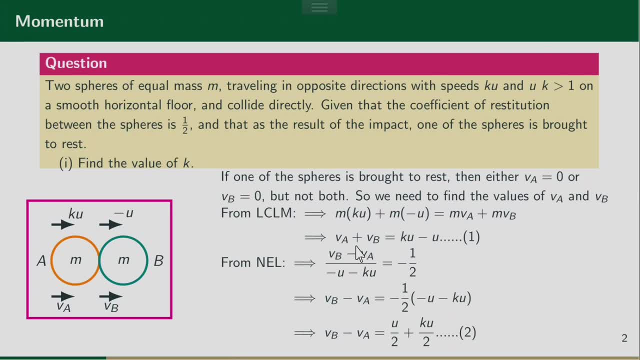 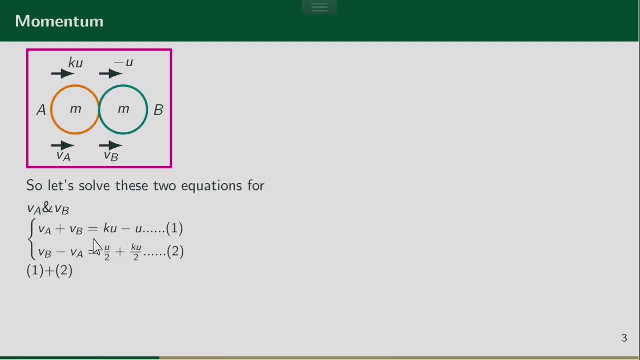 So let me call this equation 2.. What I'm left to do is to solve this equation 1 and equation 2 simultaneously, So let me write down the two equations so that I can solve them simultaneously. Now notice that I'm looking for VA and VB, so that at the end I can see which of them is 0.. 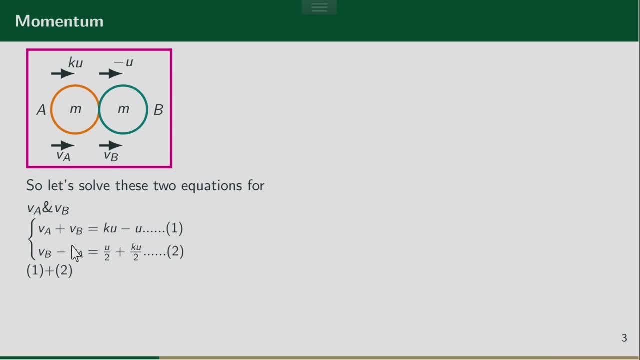 So if I add equation 1 with equation 2, the terms in VA will vanish, because of course they have the same coefficients but different signs, So VA vanishes. Then I'll be having: 2VB is equal to. I just add the right hand side, which is KU minus U. 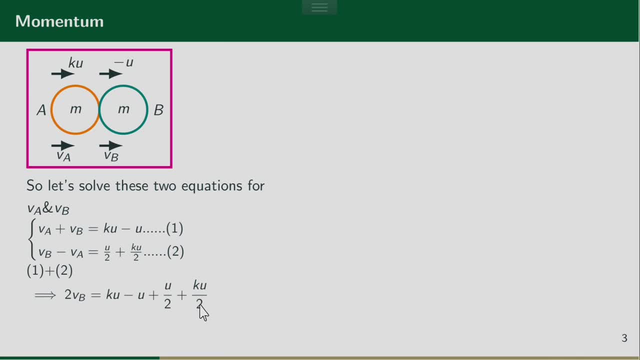 I add U on 2 plus KU divided by 2.. Let me just bring like terms together. These are terms in KU, So the coefficient of this term, The coefficient of this term, is 1 and that of this term is half. and 1 plus half gives 3 divided by 2.. 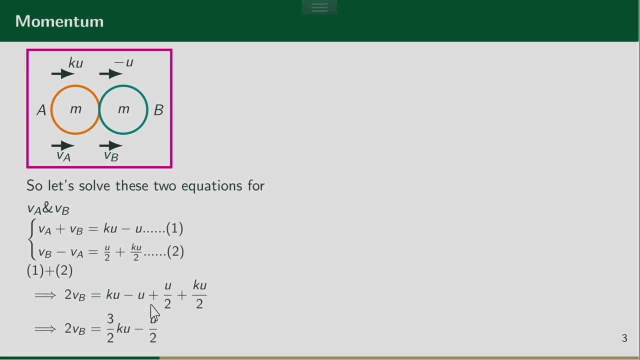 Then, in the same way, the coefficient of U here is negative 1 and that of U is half, and negative 1 plus half gives us negative half. So this is what I have. The two terms share the same denominator. I can maintain that 2VB is equals to 3KU minus U divided by 2.. 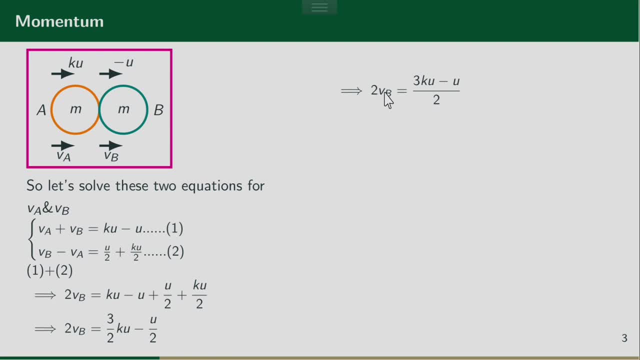 And I can now Divide both sides by 2, or I multiply each term by half. The 2 multiplies 2 and gives me 4.. So VB is 3KU minus U divided by 4.. Of course I can factor out U from these two terms and I have: VB is U into 3K minus 1 divided by 4.. 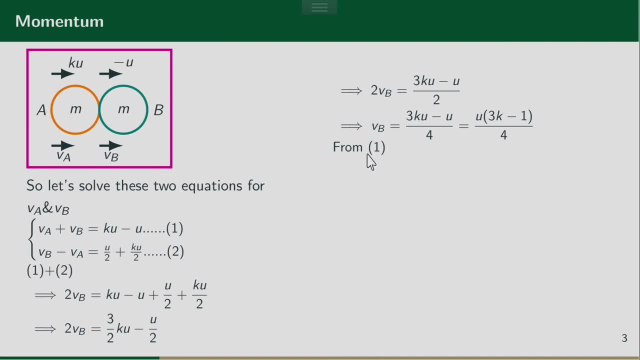 So this is a final velocity of B. Then if I go back to equation 1, I can make A the subject of VA, the subject in equation 1.. And VA will be equal to KU minus U. Then I send VB the other way and I have minus VB. 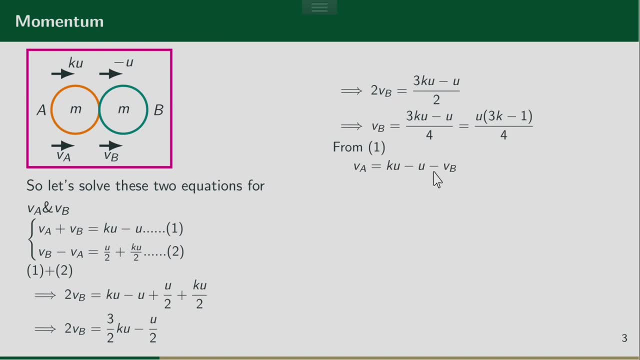 So I know the value of VB. Let me just substitute and simplify everything to obtain VA. When I substitute, I have this: Remember: this negative sign would distribute amongst all the terms in this numerator. So when I distribute, this term becomes negative and this other term becomes positive. 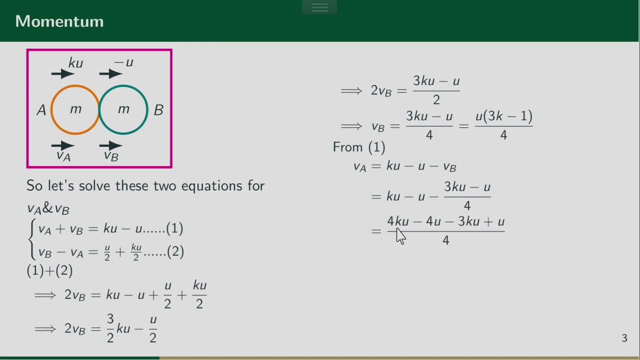 So I have this. So I will just find the LCM and distribute the terms. Then I will be having 4KU minus 3KU gives me just KU and negative 4U, 3U divided by 4.. 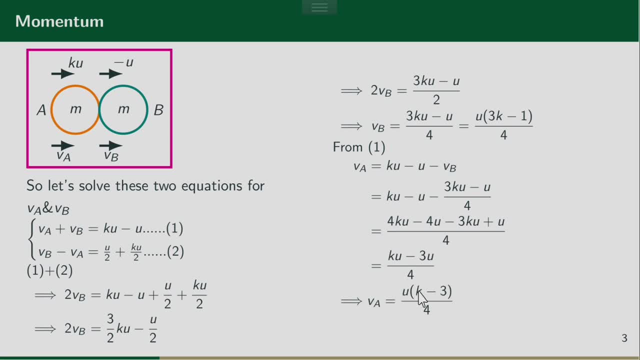 So this is the value of VA. So VA now will be U into K minus 3 divided by 4.. So I have had the value of VA and VB. Remember, in the question we were told that one of these spheres is vertical. 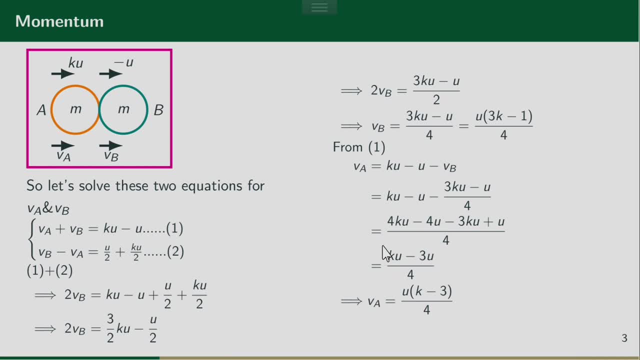 So we are going to solve for the final velocity of VA to rest as a result of the impact. So if I suppose that VB is brought to rest, that means its final velocity should be 0.. And in the case where VA is brought to rest, its final velocity 2 is 0.. 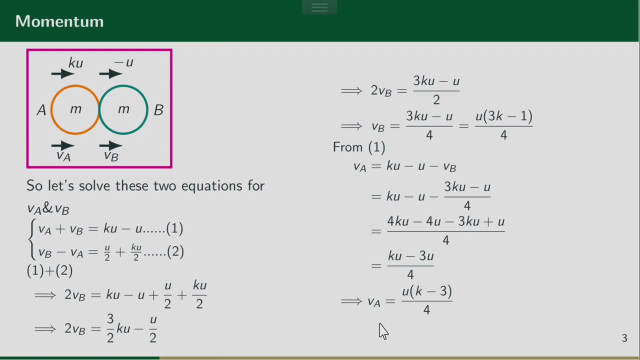 So I will just equate both VB and VA to 0 and solve for the value of K. When I am solving for K, I will go back to the premises in the question, where I was told that K is a value greater than 1.. 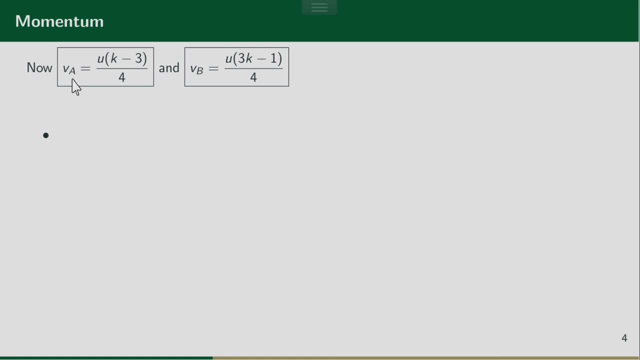 Now this is the value of the final velocity. So it is the final velocity of object A and the final velocity of object B. Now let's suppose that VA is 0. So I will take this term and equate to 0.. 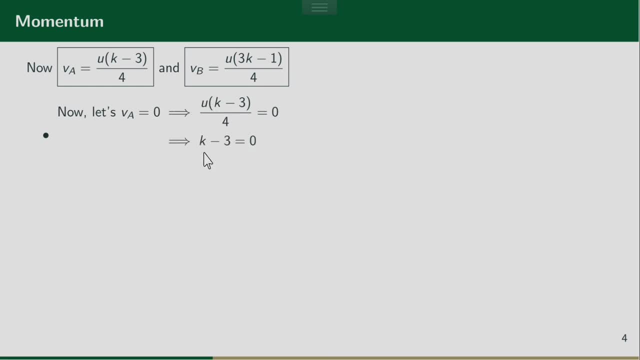 Then U divided by 4, I can divide both by U over 4. It vanishes. So K minus 3 is equal to 0. So I send negative 3. the other way, K is equal to 3.. 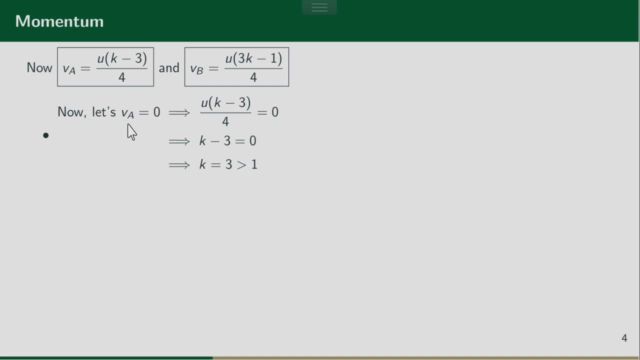 And 3 is a value which is greater than 1.. So, indeed, the final velocity of A is 0.. So A is equal to 0. So I send negative 3 the other way, So A is equal to 0.. 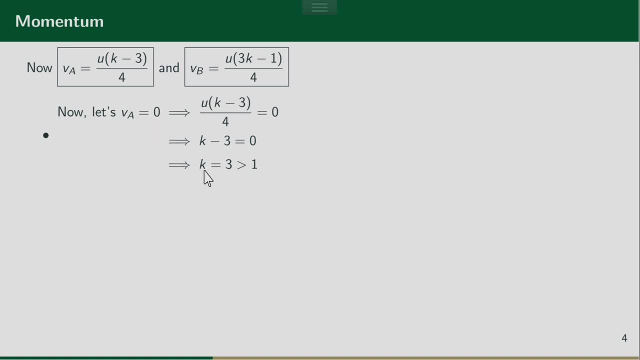 a sphere that is brought to rest because the value of k satisfies the premises that was given in the question. but let us try for vb and c now. let's suppose that vb is equals to zero. that means we will take this and equate to zero and solve. we do the same thing. we divide both sides by u on four. 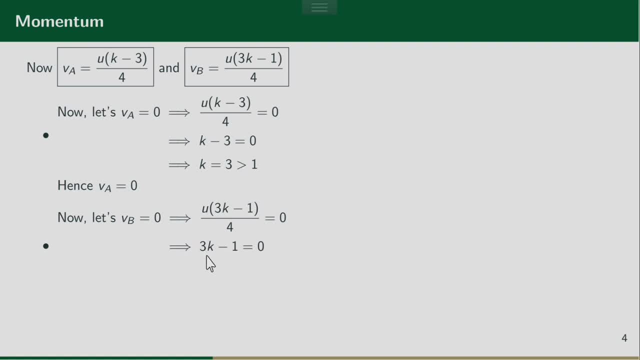 so i have three: k minus one is equals to zero, and k will give me one third, and one third, of course, is less than one. so it means the final velocity of b is not zero, so b is not brought to rest. now. the next part of the question was that let us find out this velocity of the other object. 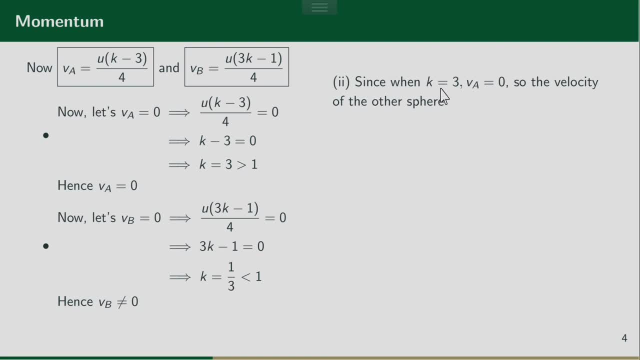 in terms of u. only we have had the value of k as three and we know that va is zero. so the velocity of the other sphere will be the velocity of vb. so i just come here and i replace k with three. so i'll be left with three into three minus one, and three times three give us nine minus. 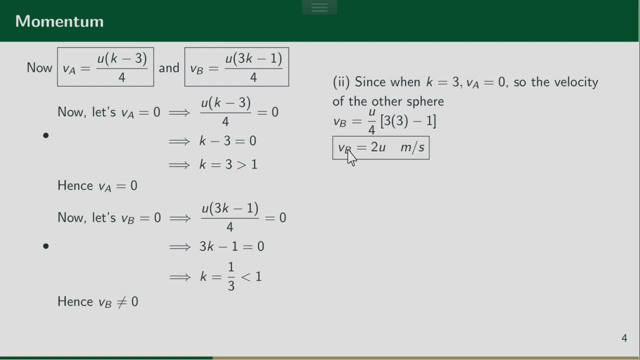 one gives eight, four goes into eight two times and the velocity of b will be two u meters per second. so i have the velocity of b. so i cannot draw. i can come back to the same figure and i write out their velocities. so instead of writing ku, i'll replace k by its value. then i go to the final velocities and a has to be zero. 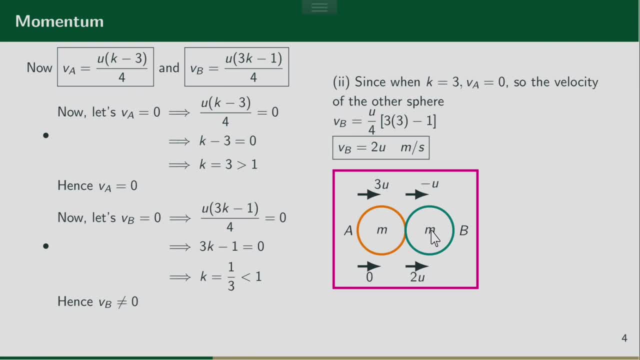 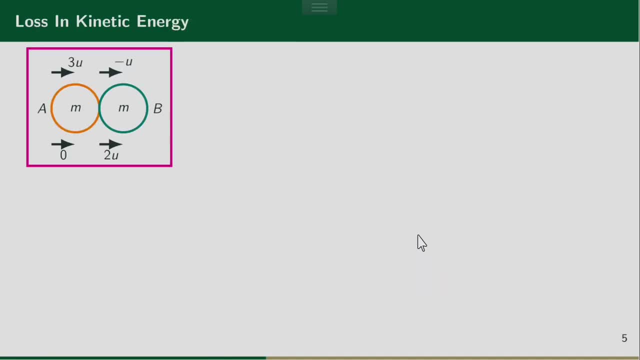 so it's final velocity is zero and b is moving with a velocity of two u after collision. so i can go ahead and solve the other question that will be asked now. the other question was that let us find the lost in kinetic energy. we know that when two objects interact, energy is lost, maybe as heat sound. 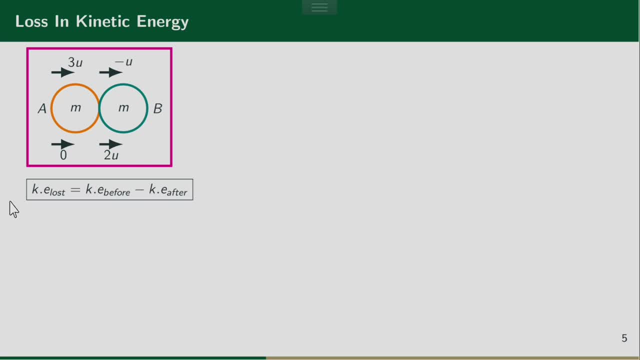 or energy of deformation. now ke loss is given by the kinetic energy of the object, energy the system had before collision. take away the kinetic energy the system had after collision, so that means ke before the ke of the object a. i added to ke of the object b. 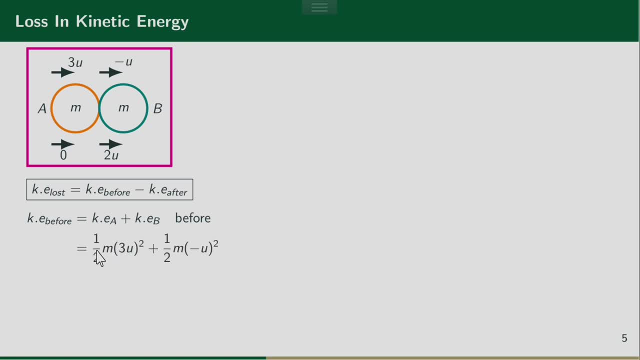 and that is before. so what is kinetic energy? half of the mass multiplied by the velocity, order squared. that's why i have half m into three u order squared, then plus m into negative u order squared. so this will give me the kinetic energy the two objects had before. 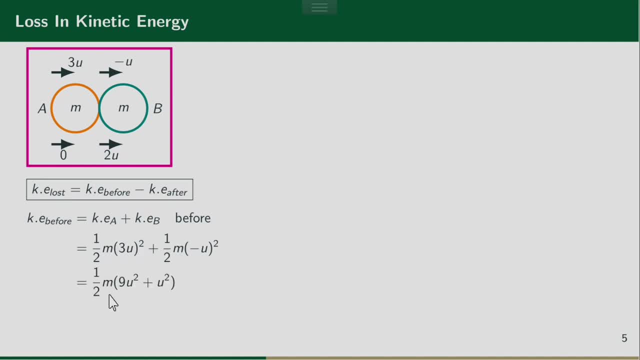 impact. so, doing the maths, i can factor out half m into plus u squared. nine u squared plus u squared give us 10? u squared, and two goes into ten five times. so simplifying everything here gives us five m? u squared. so this is the kinetic energy of the body. 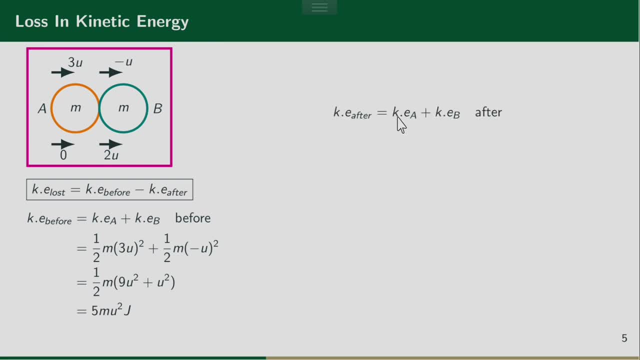 before collision. now what about after? after would just be the ke that each of the objects have, but after impact. so i just find the kinetic energy of each of the particles, but of course the kinetic energy of the sphere a after impact is zero, because after impact is brought to rest and it is not moving, so it has. 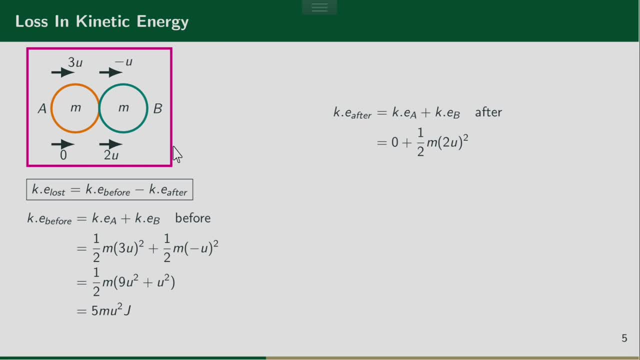 no velocity now. so the only kinetic energy after impact will be the ke of the sphere b. so we just find the kinetic energy of sphere b, which is half m into into two? u order squared, which give us half m into four? u squared, two goes into four two times, which give us two m? u squared.